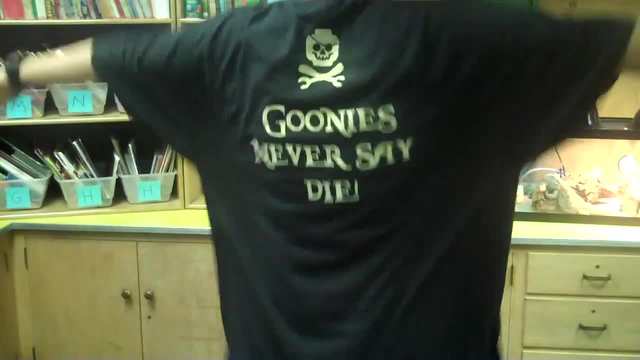 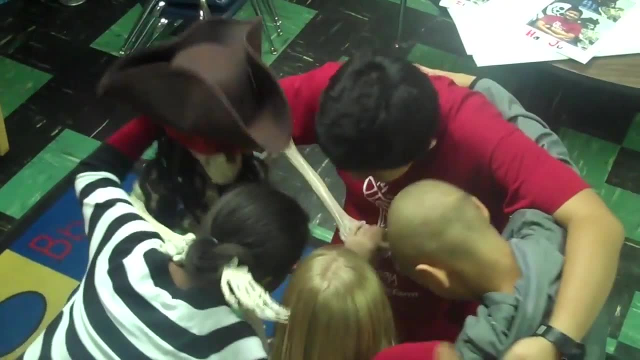 We're the Goonies, and the Goonies never say die, No, we don't. Today we'll build the alligator with a motor and some pulleys. We'll put our heads together. Yeah, we're smarter than the pulleys. 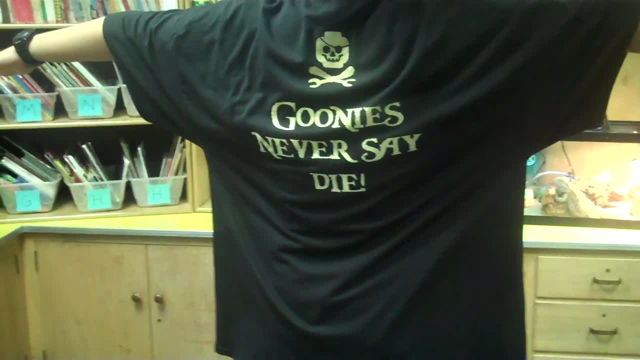 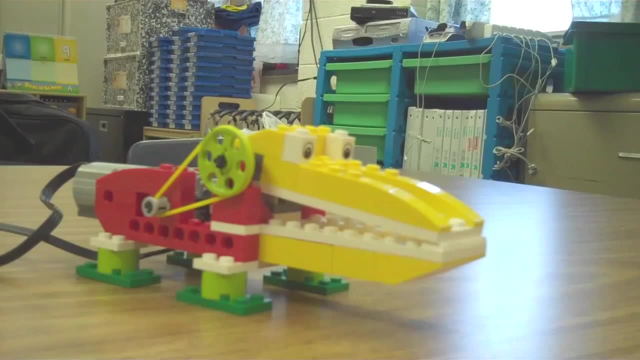 We're the Goonies, and the Goonies never say die. These are all the pieces you will need to build this model. Don't worry, you don't have to memorize all these pieces, And this is what your alligator will look like when it's done. 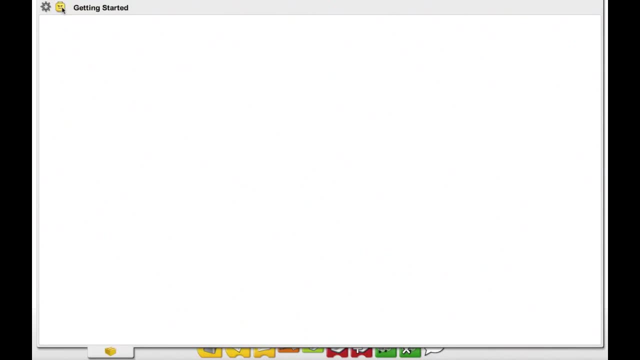 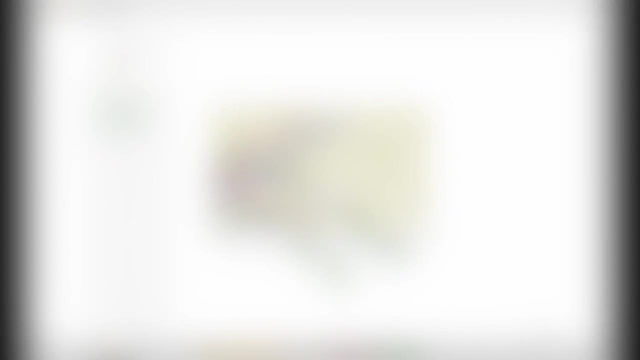 When you open the model, you'll see that it has all the pieces you need To open the We Do software. this is where you'll find the step-by-step building instructions. Choose the model you want to build and watch the video if you want, and then follow the step-by-step directions on the screen by clicking on the forward or back buttons. 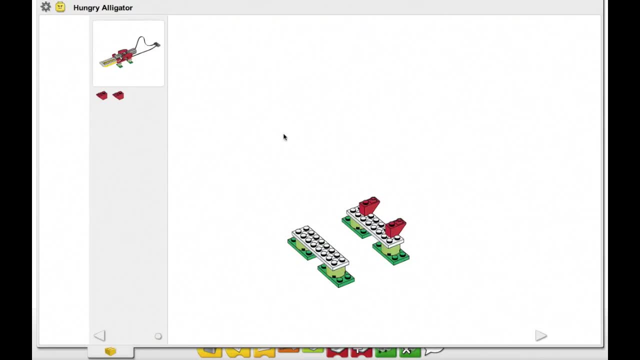 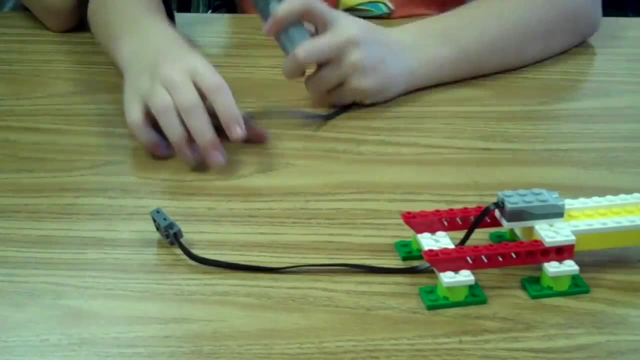 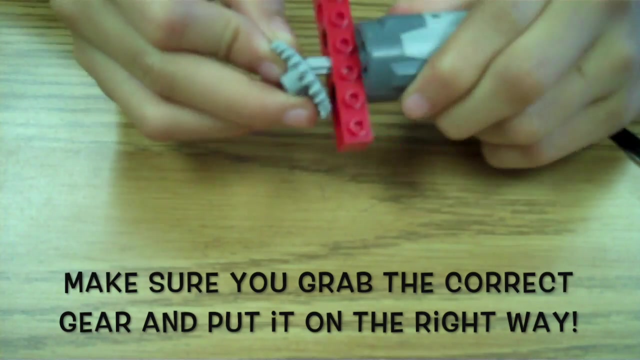 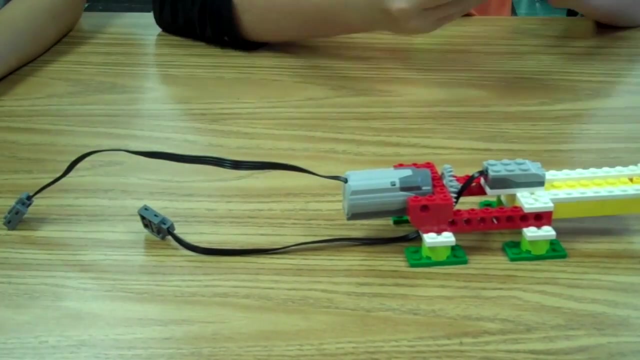 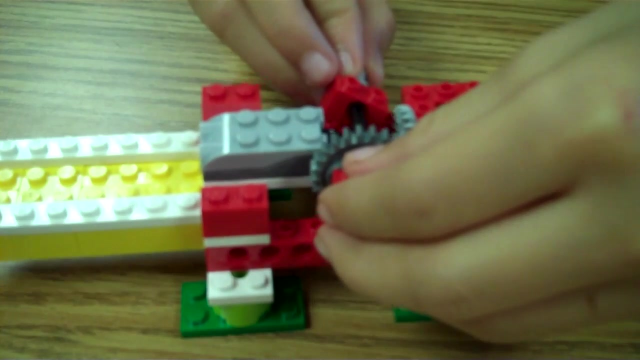 This one takes you to the next step, and this one takes you back a step. So here's how you build it. Here's how it looks like. Make sure the red bricks are as far apart as they can be before you try to attach this part. 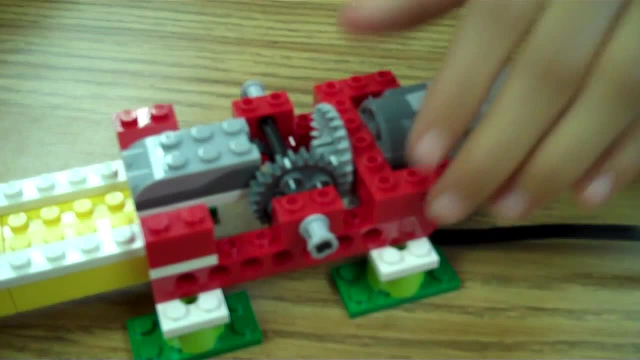 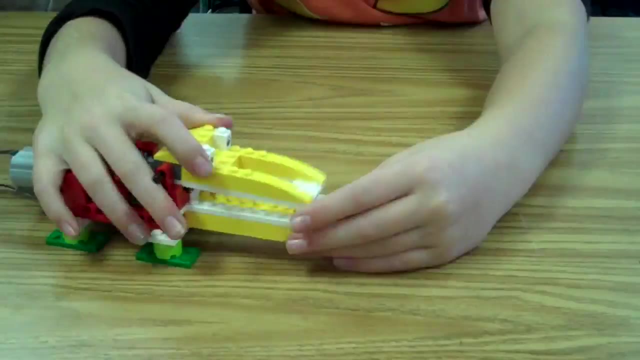 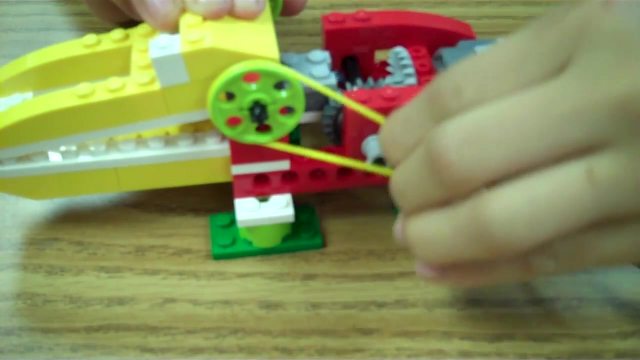 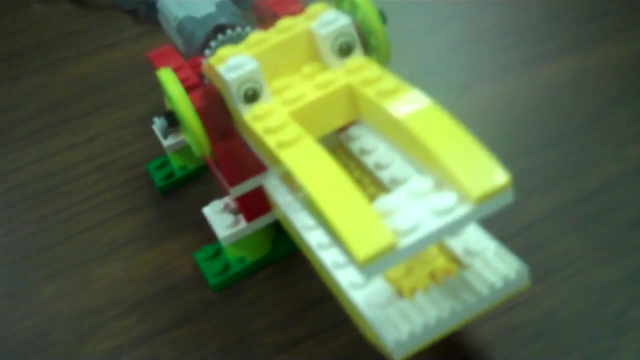 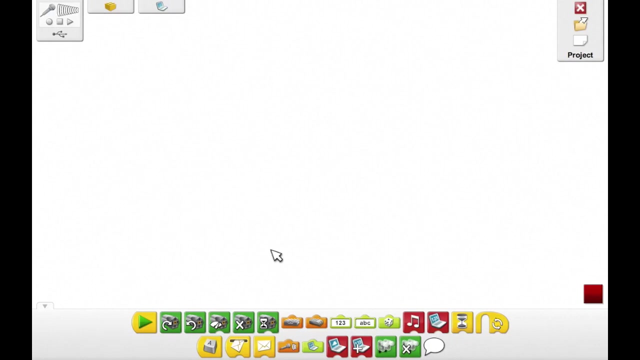 It should look like this. We found it easier to attach the rubber bands when you start by attaching it to the green pulley. This is how it looks once you've built it. First, you find the start button and drag it out onto the white space. 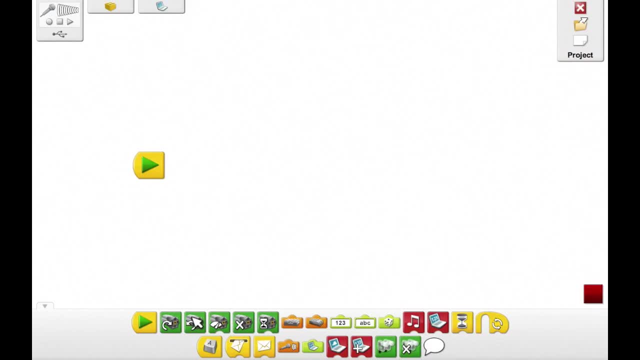 When you click on this button it will start the program you create. Next, drag the motor that way, block and connect it to the start button. This will tell the alligator to open its mouth. Then drag and connect a motor on for block and type a 5 into the box.